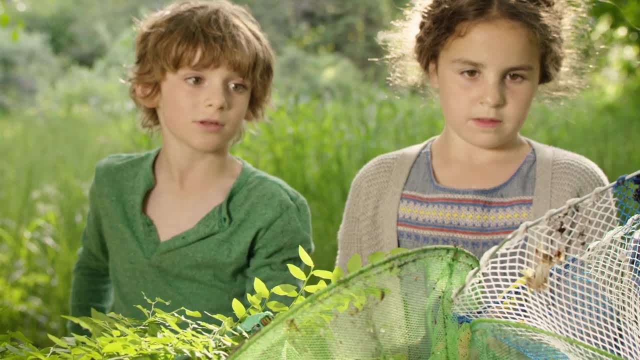 Look, That's a frog. Hi froggy, Hi froggy. Well done nature detectives. Now let's connect the clues to solve the mystery. Now let's connect the clues to solve the mystery. You found a marsh with some lilypads and a frog. 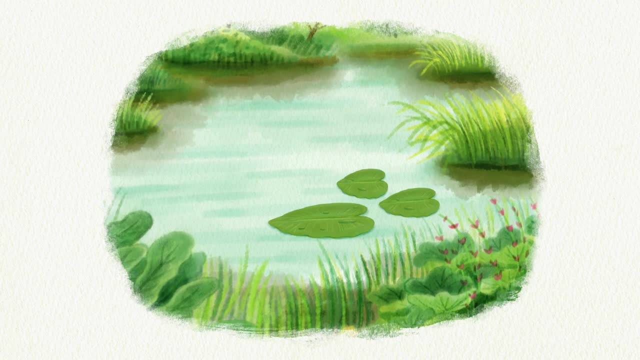 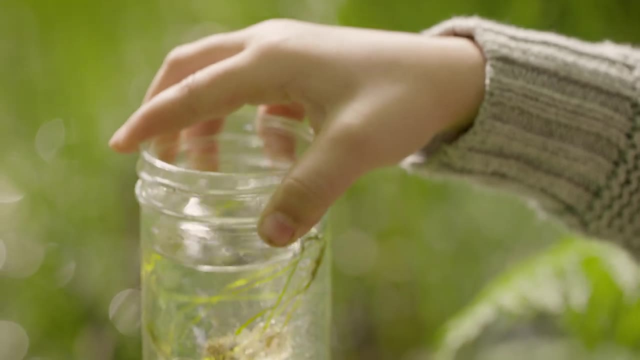 You found a marsh with some lilypads and a frog. Now, what's with this spotted jelly? Now, what's with this spotted jelly? Now, what's with this spotted jelly That looks like jelly. That looks like jelly Nearly there. Gumboot Kids. 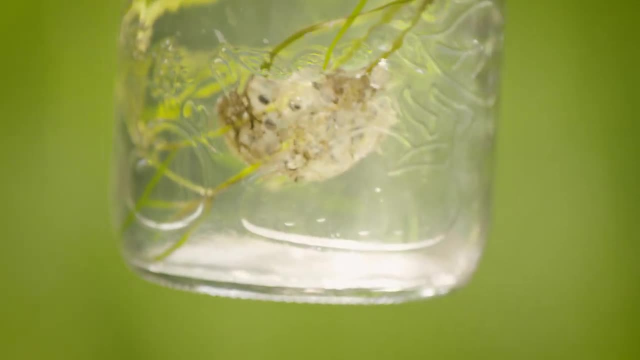 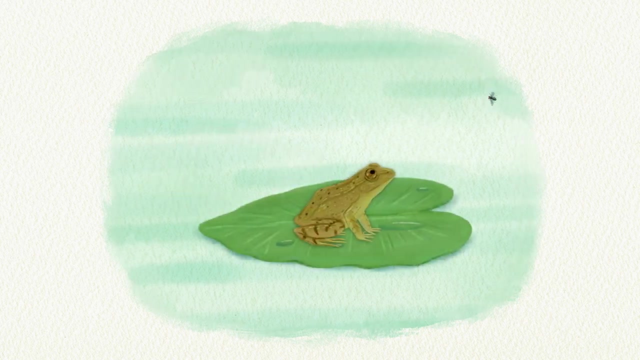 I see black spots, But what are they? Those spots are going to grow into jelly. Those spots are going to grow into tadpoles, And those tadpoles will grow into, I know, frogs. So the spotted jelly must be frog eggs. 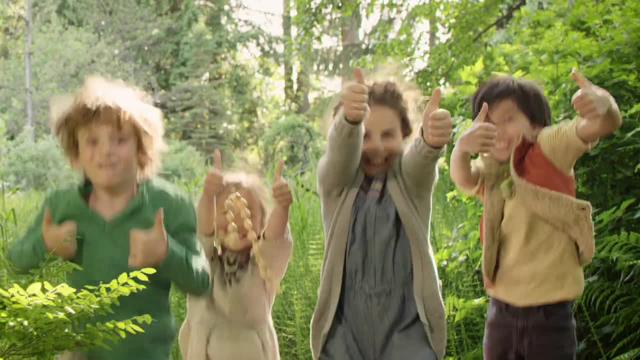 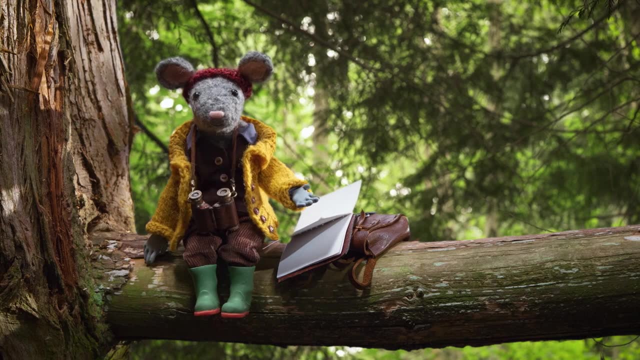 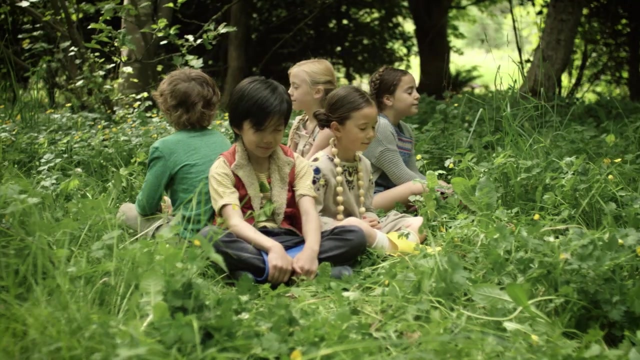 That's right, We did it. Case closed. Yay, Way to go. Now let's pause and have a mindful moment. Notice how frogs sit so still and alert. Notice how frogs sit so still and alert. Try sitting still like a frog. 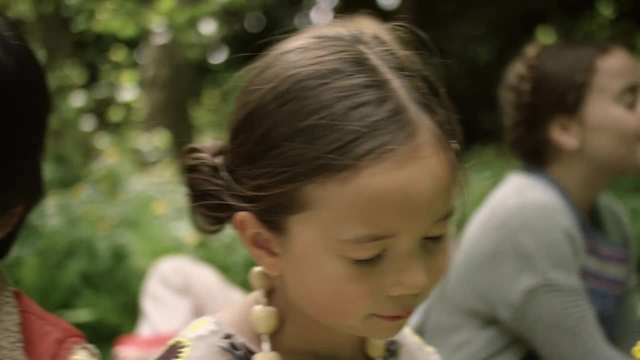 Cross your legs and place your hands on your knees. Cross your legs and place your hands on your knees. Sit slowly in through your nose and out through your mouth. Sit slowly in through your nose and out through your mouth. Frogs can sit still for a long time. 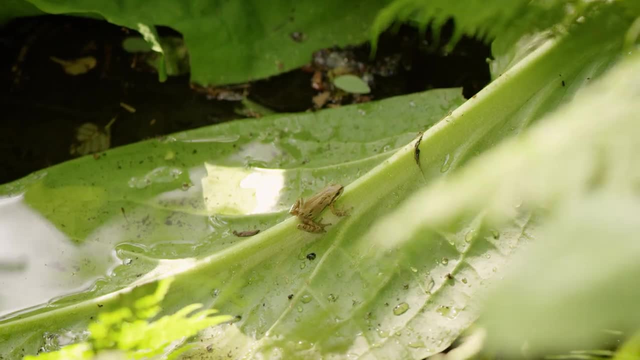 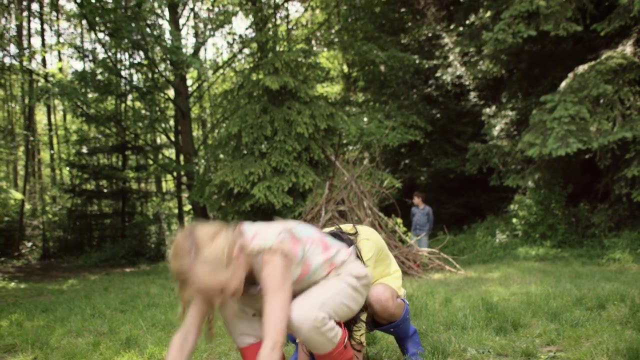 Frogs can sit still for a long time. Then suddenly hop, I just want to be a frog. I just want to be a frog Sitting here on a log. Sitting here on a log, Flicking my tongue at flies, Croaky voice and big round eyes. 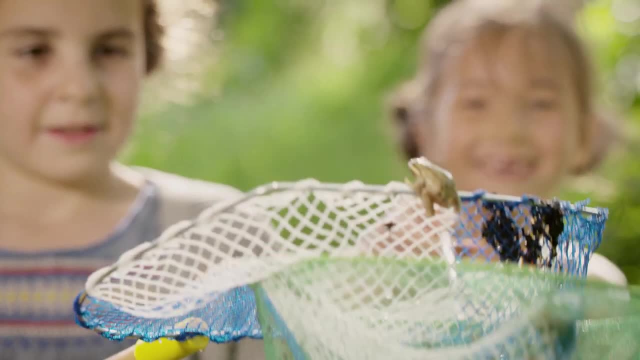 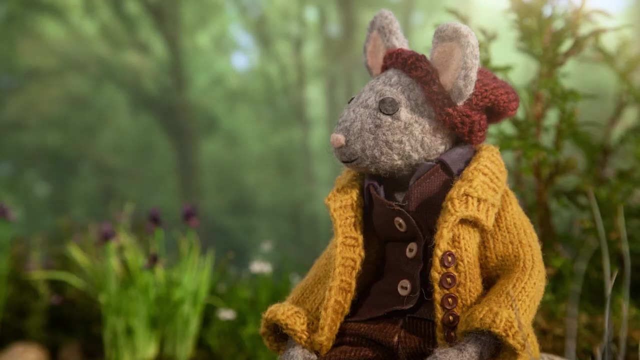 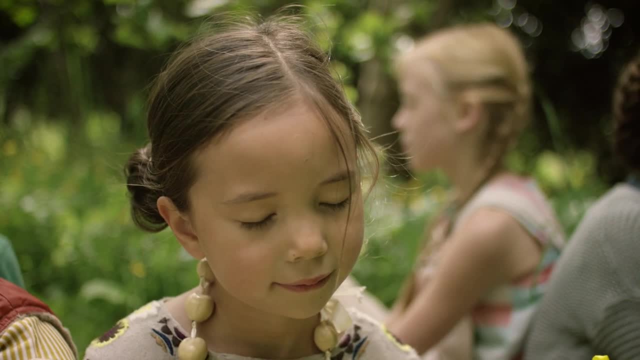 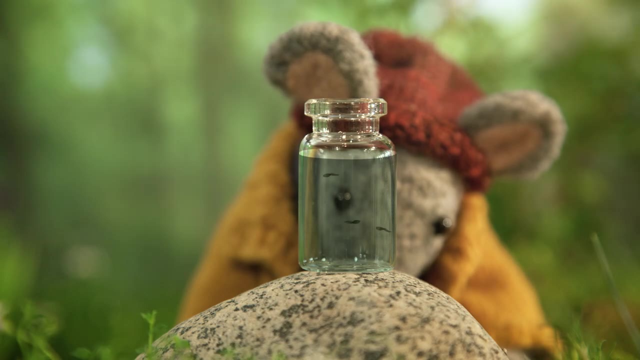 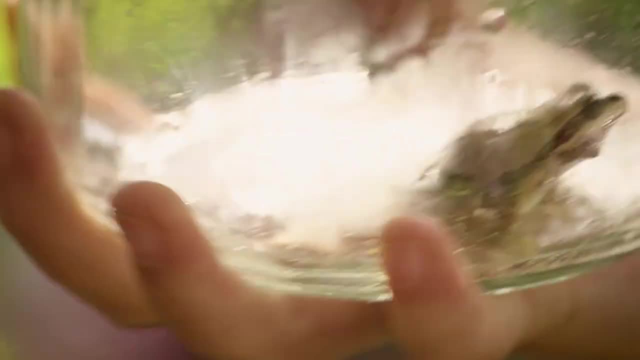 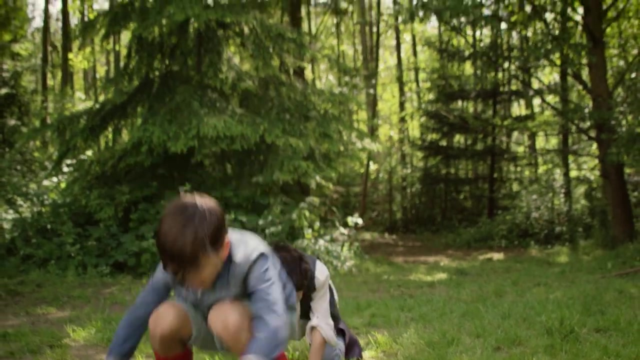 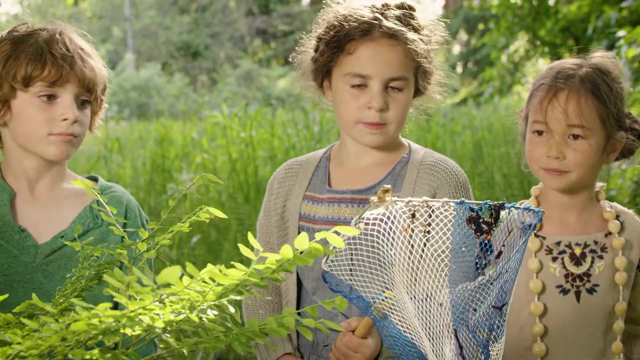 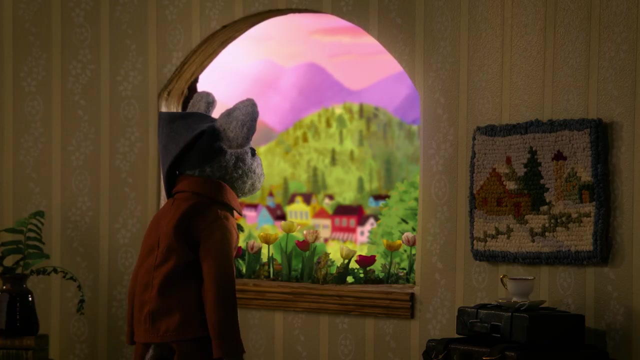 I just want to be a frog, Happy in a big old bog, Leaping from the lily pad. Warming sun ain't so bad. I couldn't dream of a better life. I couldn't think of a better life. Ah, it's amazing. those little spots grow up into frogs. 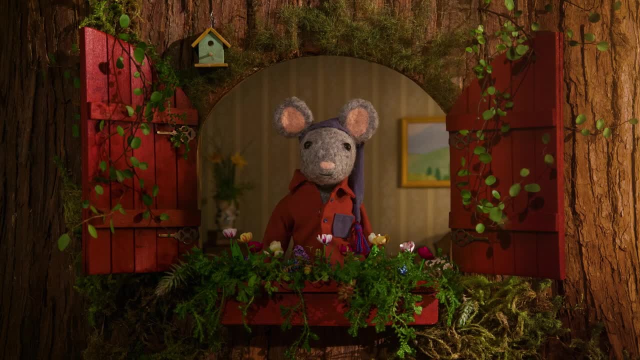 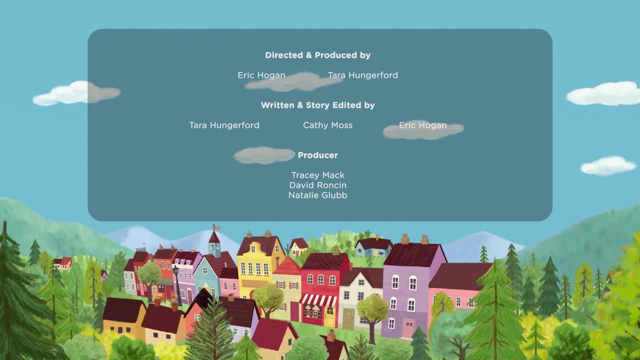 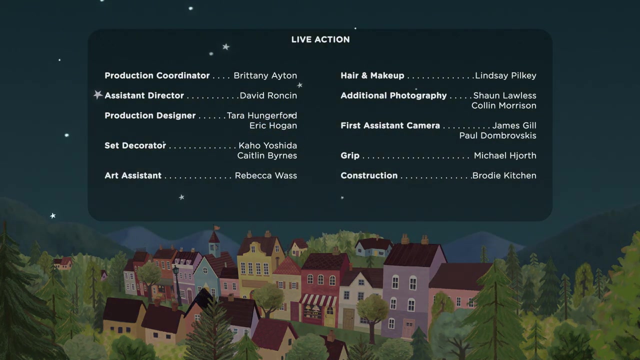 Hear that Sounds like our frog friends are saying goodbye. Good night Gumboot Kids. Good night Scouts. Na-na-na-na-na-na, Na-na-na-na-na-na, Na-na-na-na-na-na, Na-na-na-na-na-na, Na-na-na-na-na-na-na. 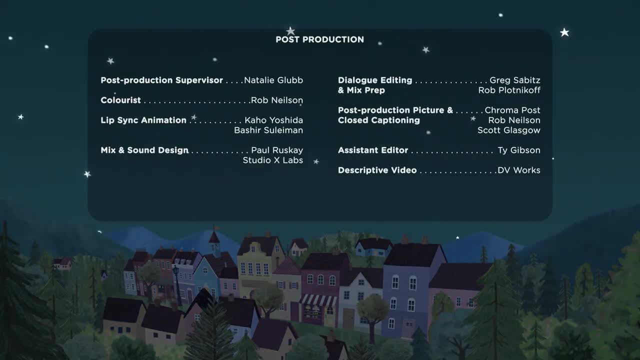 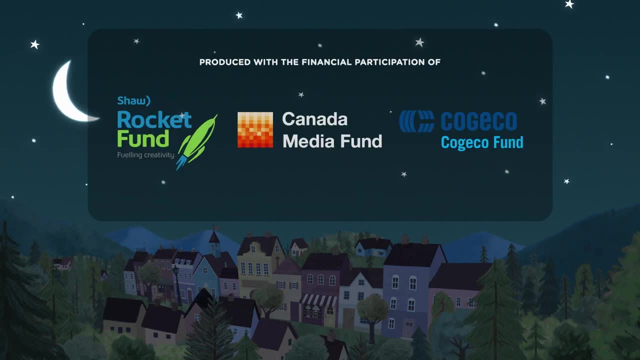 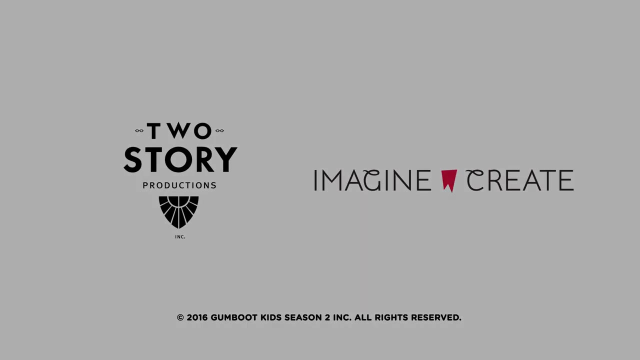 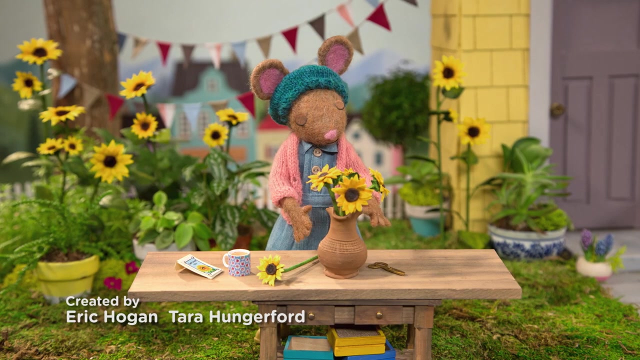 I couldn't dream of a better life. Na-na-na-na-na-na-na, I couldn't dream of a better life. I couldn't think of a better life. Meet Daisy. she's got a way of making beautiful things. You never know what nature will teach her. 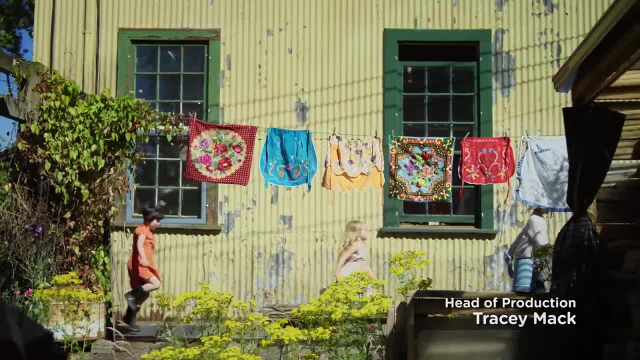 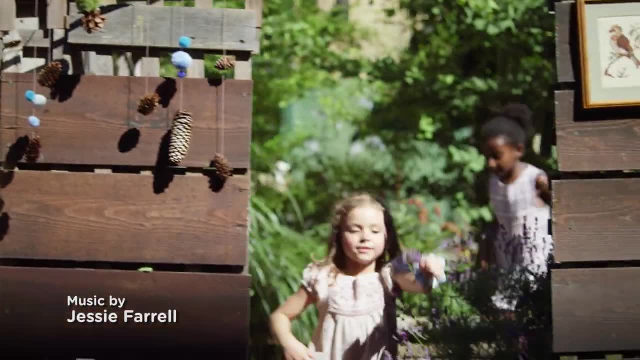 What inspiration will bring D-O-Y D-O-Y Daisy? What are we making today? D-O-Y D-O-Y Daisy. D-O-Y D-O-Y Daisy, D-O-Y D-O-Y Daisy. I bet we'll make something great. 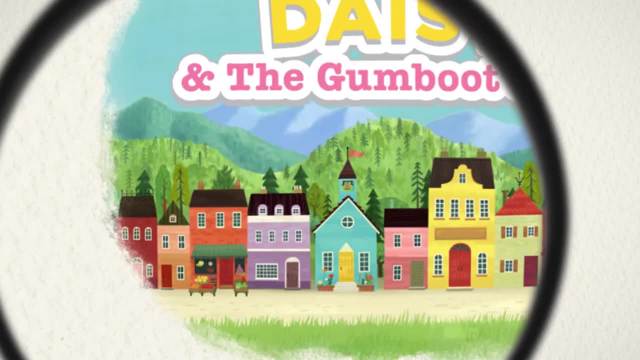 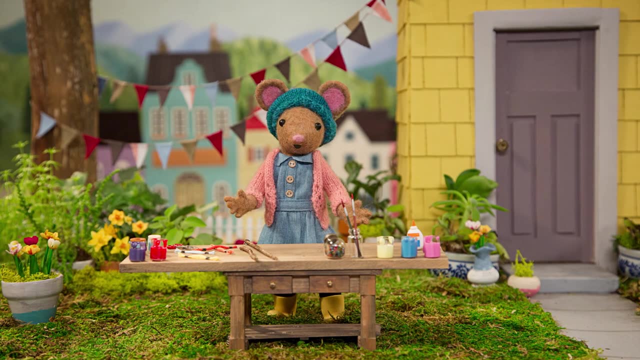 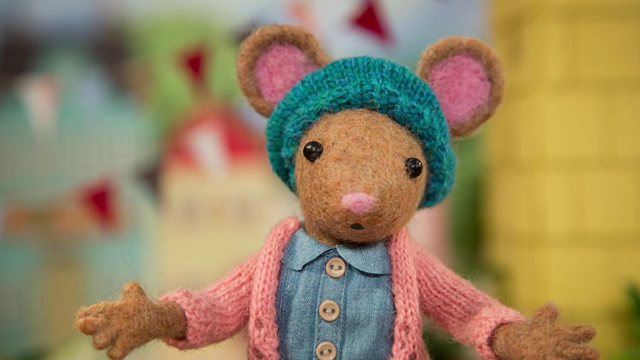 Hello Gumboot Kids, Hi Daisy. I love walking by the pond in the park. Just this morning I was so excited to see all kinds of pond creatures like minnows, turtles, dragonflies and- my favorite frogs. 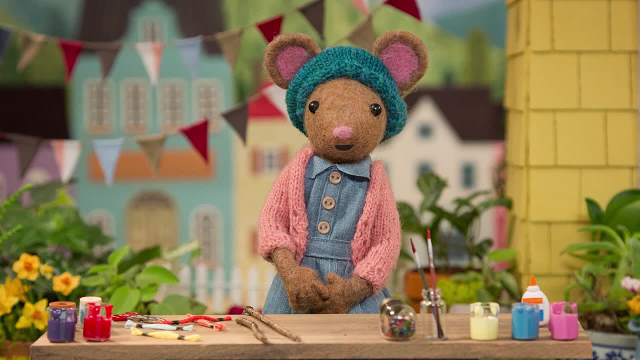 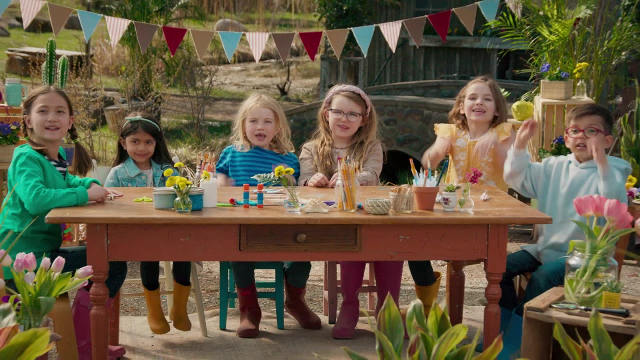 They were leaping from lily pad to lily pad. Ponds are fascinating places to find inspiration. Would you like to make some clothes peg pond creatures with me? Gumboot Kids- Yay, All right, let's do this. Step one. 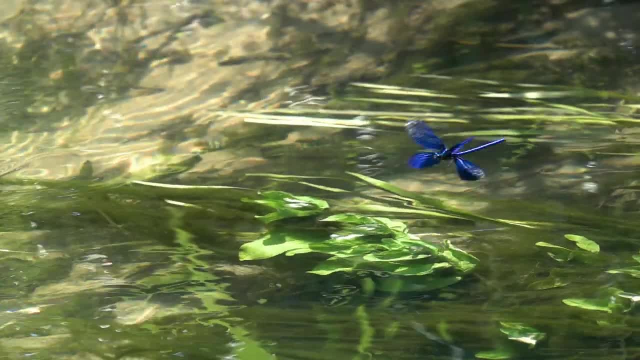 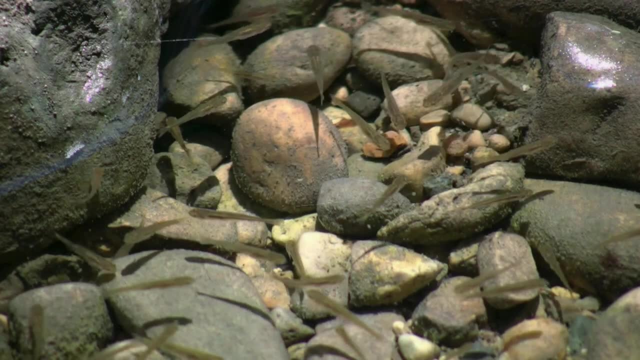 Let's observe some pond creatures. Lots of different creatures live in and around ponds. What pond creature would you like to make? I'm going to make a worm. I'm going to make a fish. I've seen frogs in the creek by my house. 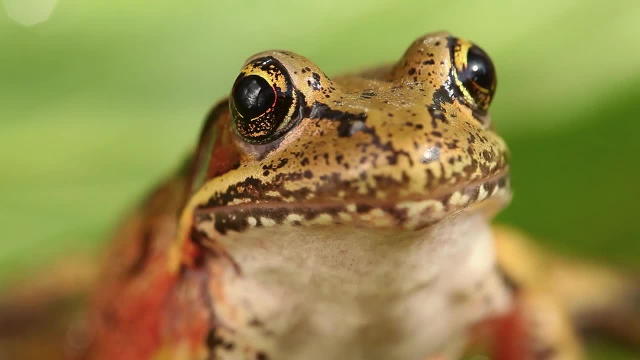 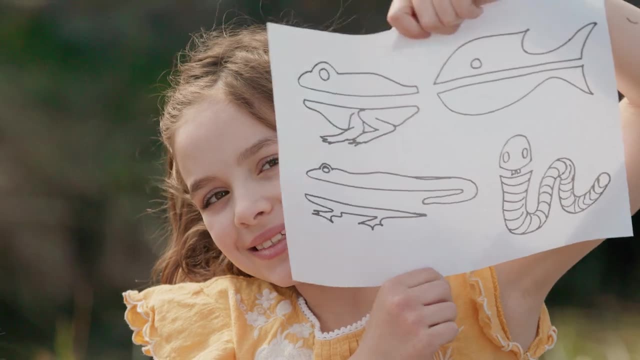 I'll make a frog. I love when they caw. I'll make a frog. Step two: Draw the outline of your creature's profile. That's it Looking good. Use a felt pen to draw features on your creature. You'll want to draw it about the length of a clothes peg. 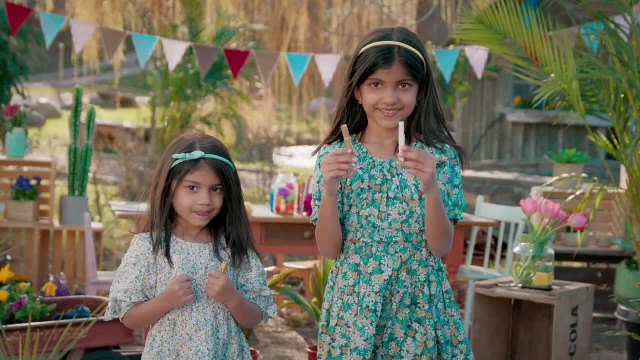 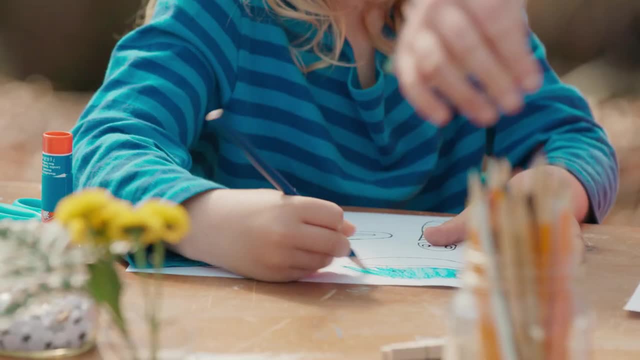 Later we'll use the clothes peg to make our creatures come to life. Great, I'm going to draw big eyes on my frog. Once you've drawn the outline, color it in. What color is your pond creature? I like bright green. 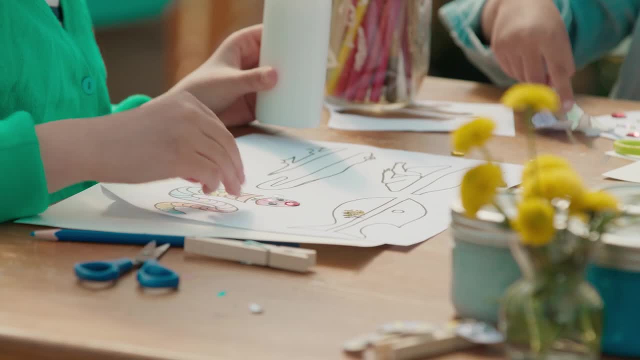 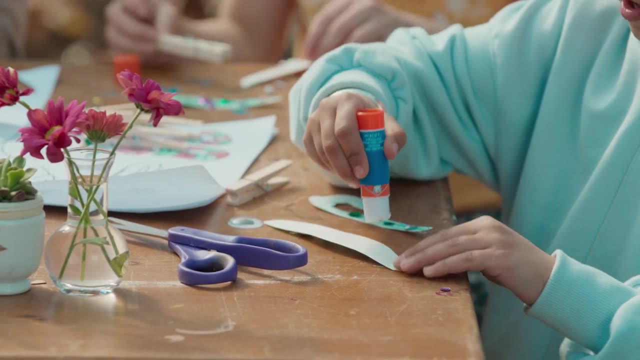 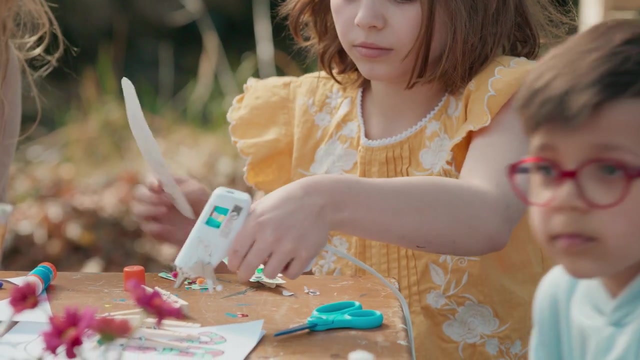 Now let's decorate. I'm going to decorate mine with shiny sequins. Step number three: Cut out your creature and glue it to a clothes peg. Line up the creature so that its mouth is at the opening of the clothes peg and the tail is at the part of the clothes peg that you pinch to open. 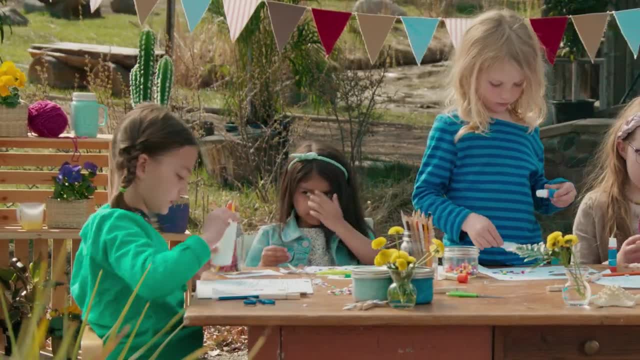 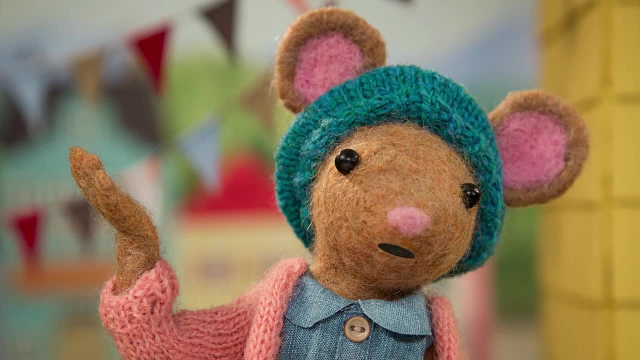 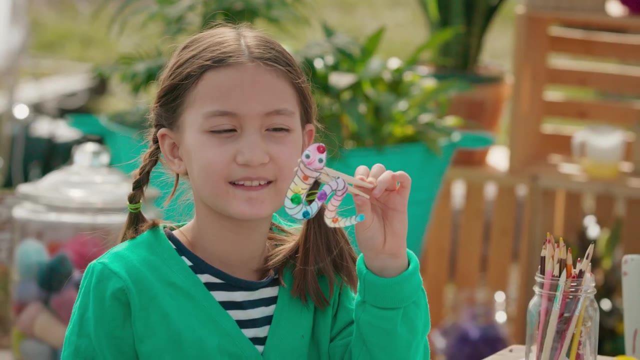 Can you please help me with the glue? Yes, of course, Thank you. I love making nature crafts. Great work, Gumboot Kids. All right, let's see what you've made. These pond creatures are so funny And cute. 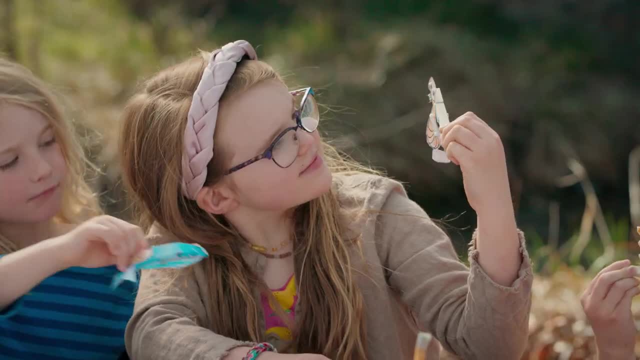 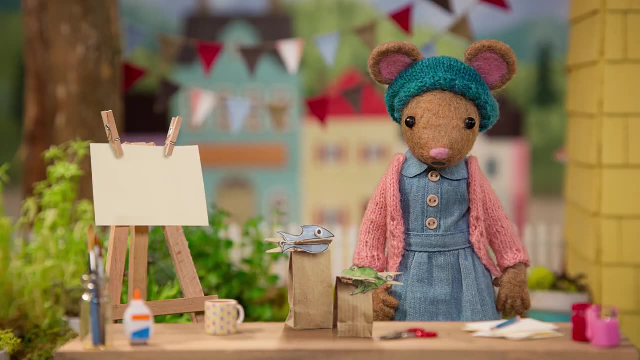 Your fish looks really good. Thank you, I like your worm. Thank you, Aww, Your pond creatures are super cute. I'm using mine to clip my papers together on my desk Like this. See you soon. Gumboot Kids. 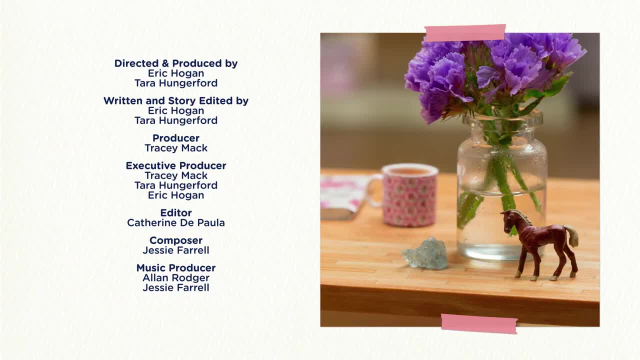 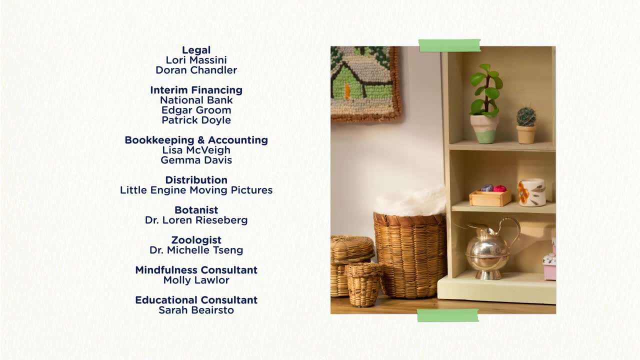 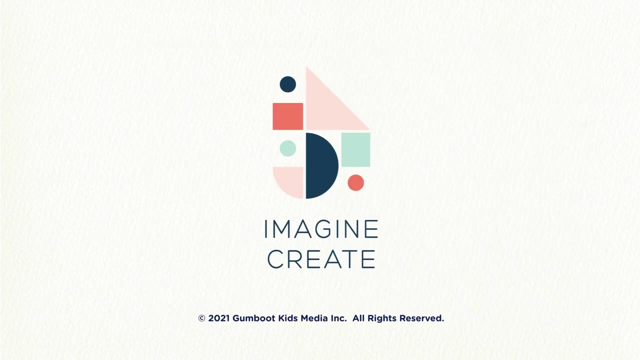 Goodbye Daisy. Bye T-O-Y D-O-Y Daisy. what are we making today? Does Swamp defer長 달라 3 Saga T-O-Y D-O-Y Daisy? I bet we'll make something great. 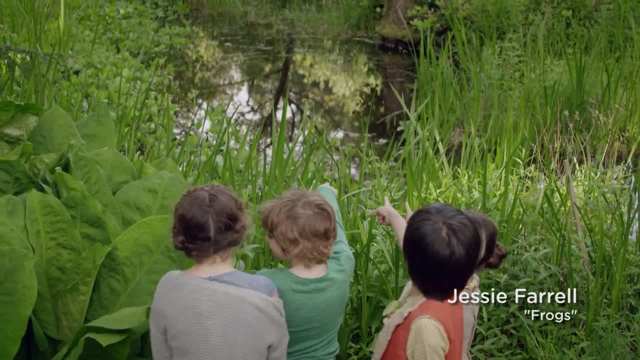 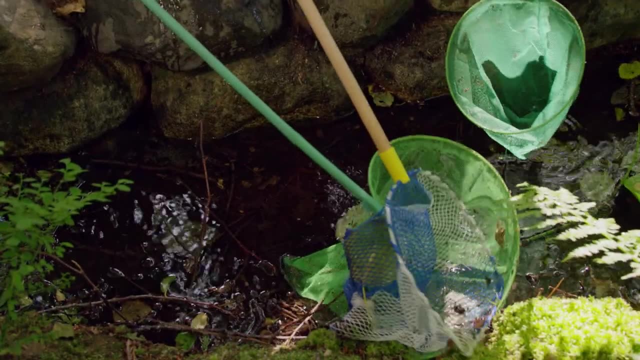 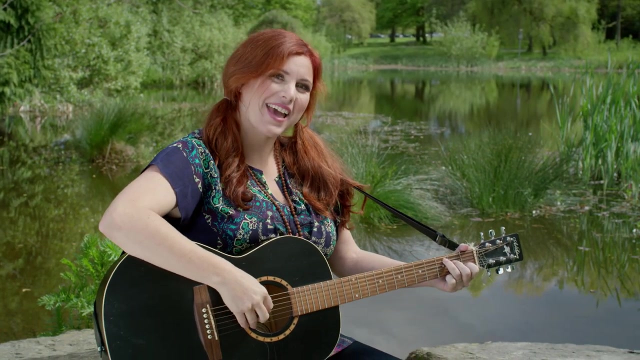